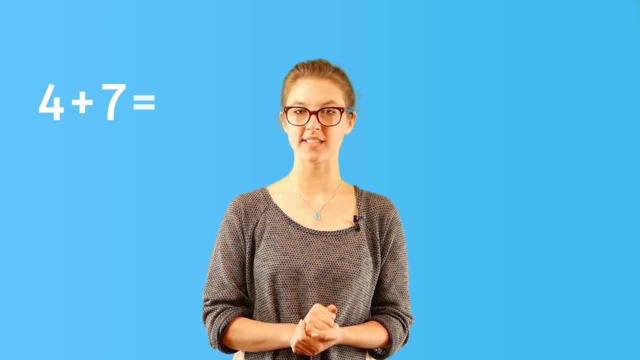 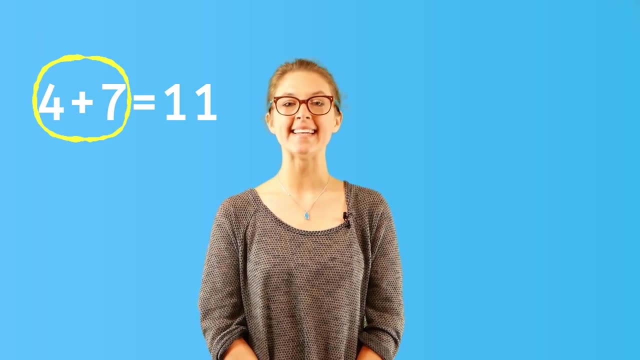 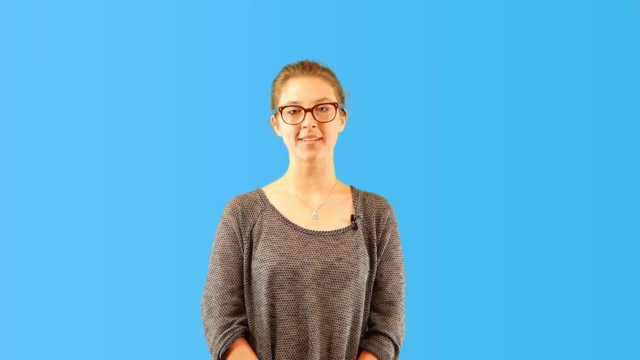 For example, 4 plus 7 equals 11.. This is a true number sentence, because what is on one side of the equal sign is the same or equal to what is on the other side. Now let's look at how to use number sentences or equations to help you solve world problems. 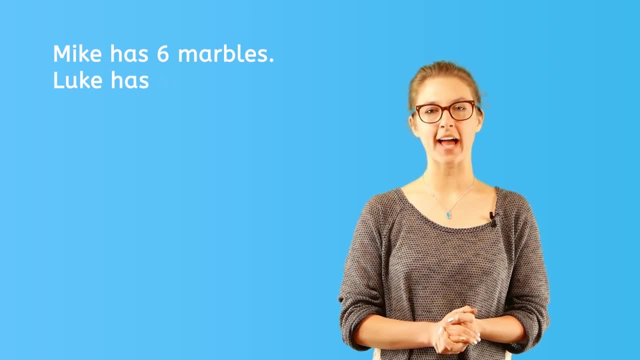 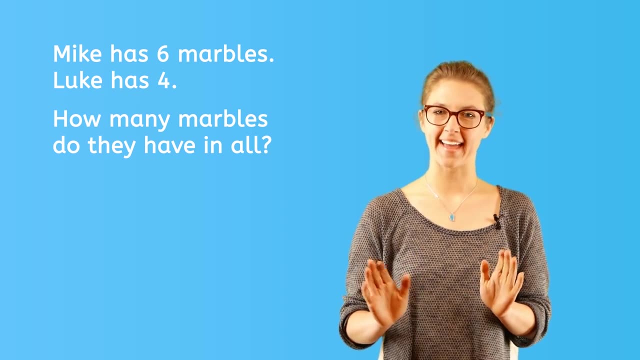 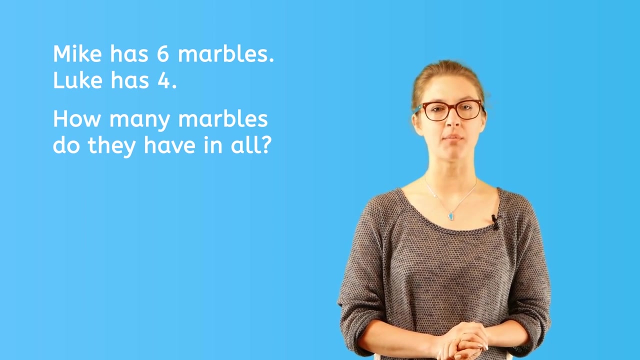 1. Mike has 6 marbles, Luke has 4. How many marbles do they have in all? Okay, so you know that we can act it all out, draw a picture or use a number line to solve this problem. 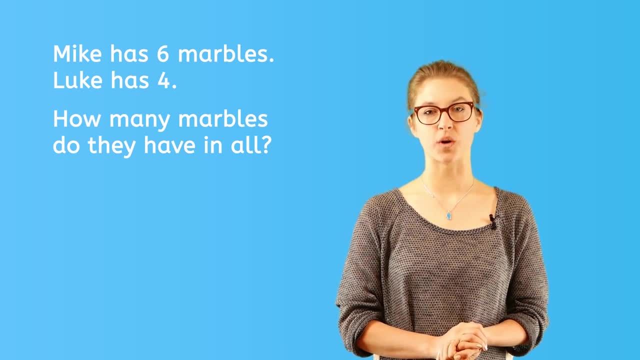 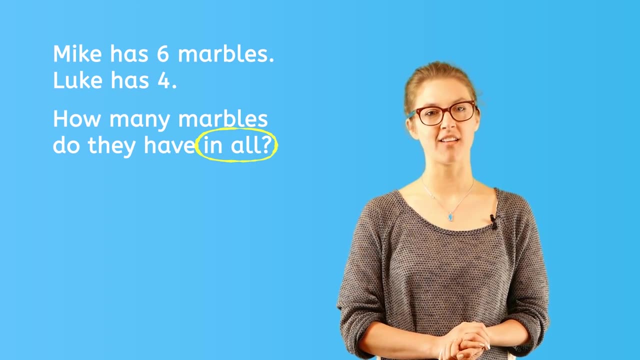 We can also skip those steps and write a number, sentence or equation right away. We know that we will need to add because it says in all: 2. The Manners mean that all the other R non-narrative materials in our problem. 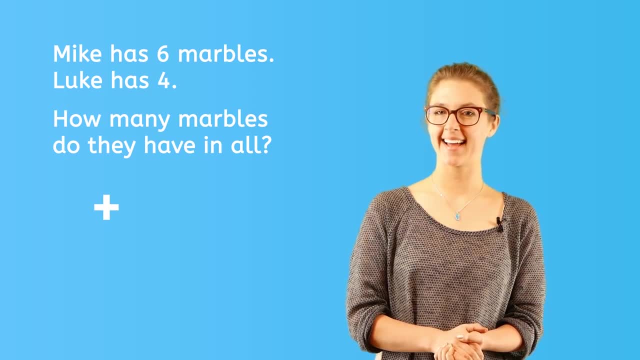 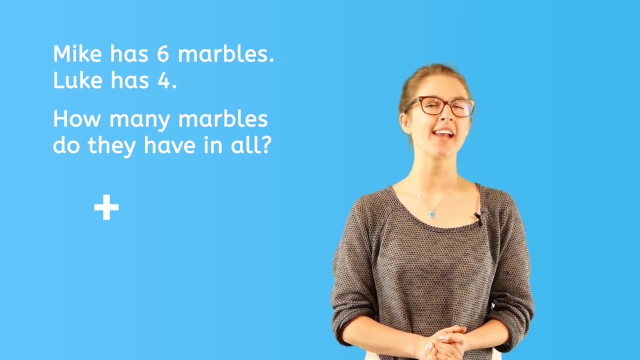 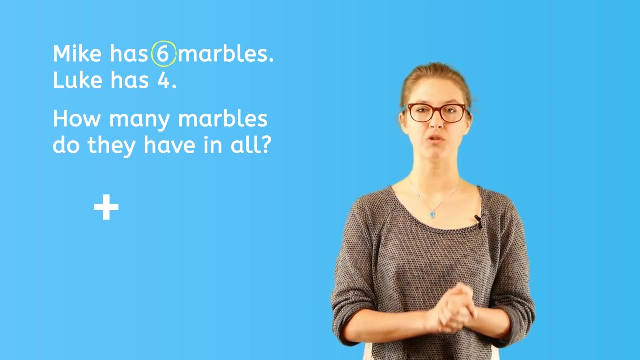 That's great, because you already know what operation symbol will be in our number sentences. What else do we know? We know that Mike has 6 marbles and Luke has 4, and we're trying to find out how many marbles they have in all. 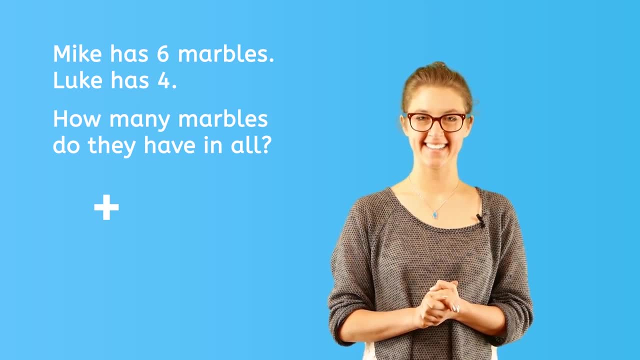 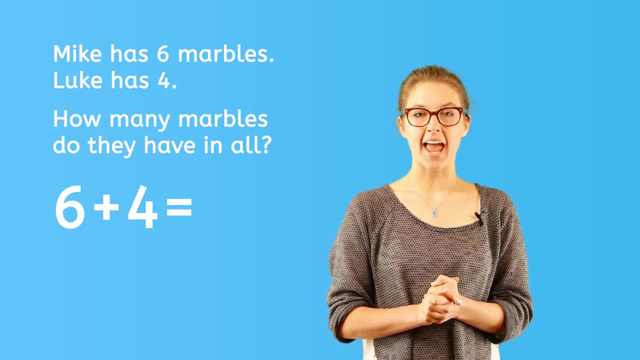 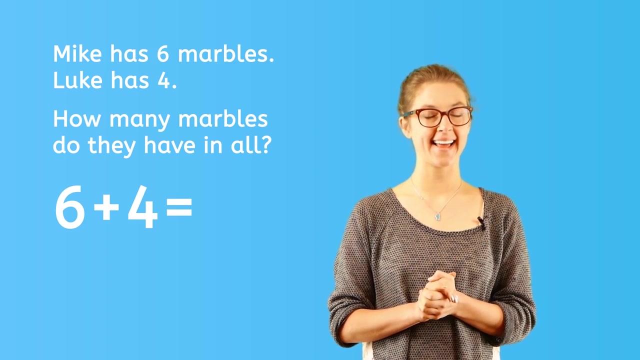 So we are adding Mike's 6 marbles to Luke's 4 marbles- Great. Now we add the equality symbol, or equal sign, and we have the equation we are trying to solve: 6 plus 4 equals. What does 6 plus 4 equal? 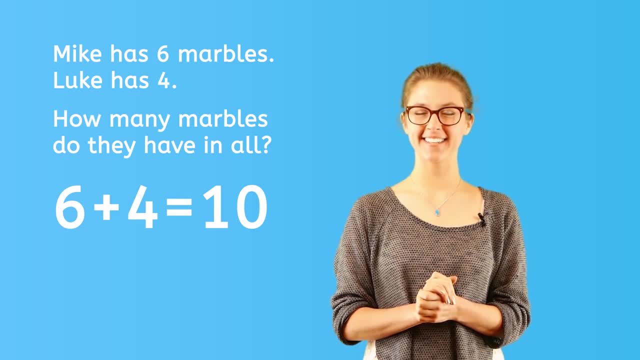 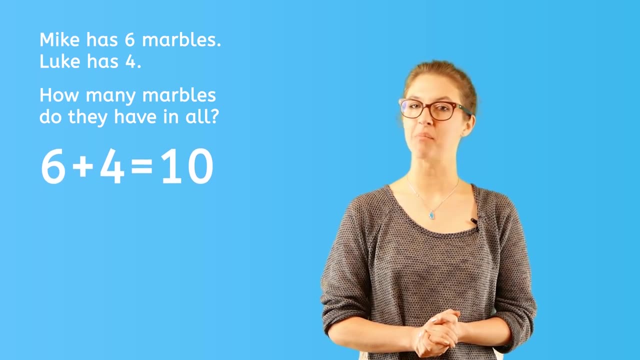 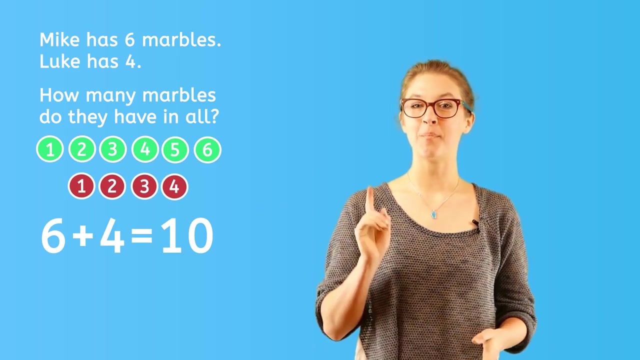 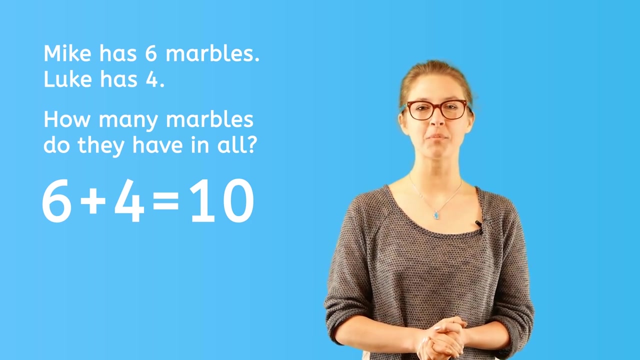 10!. You got it Good job. Sometimes you will find that it is easier to first act it out, draw a picture or use a number line before writing a number sentence. That's perfect. You can do both, But if you're ready to skip the first step, you can go straight to writing number sentences or equations when solving word problems. 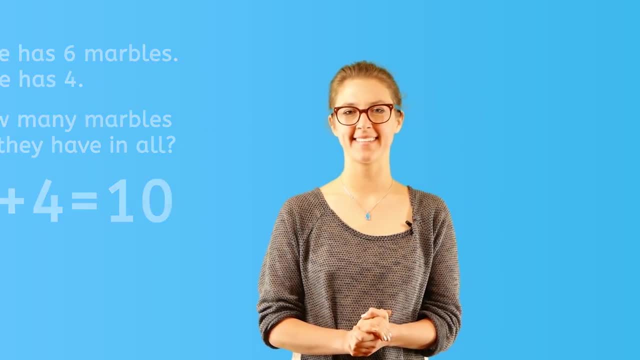 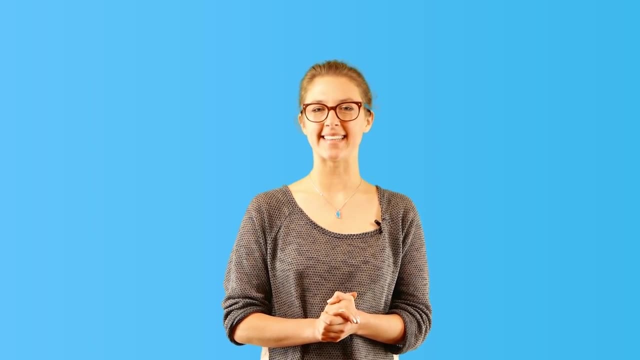 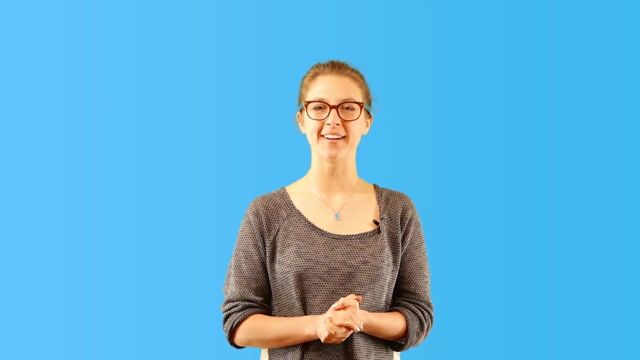 Use what works best for you. And there you have it: Another problem-solving strategy under your belt. You can keep practicing this and all other math problem-solving strategies on our fun online games and quizzes, And don't forget to subscribe. And remember, always be clever.